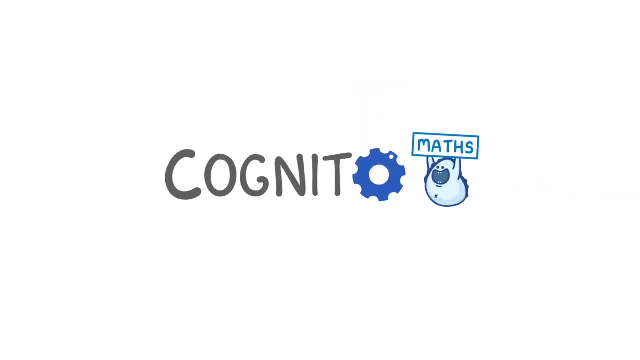 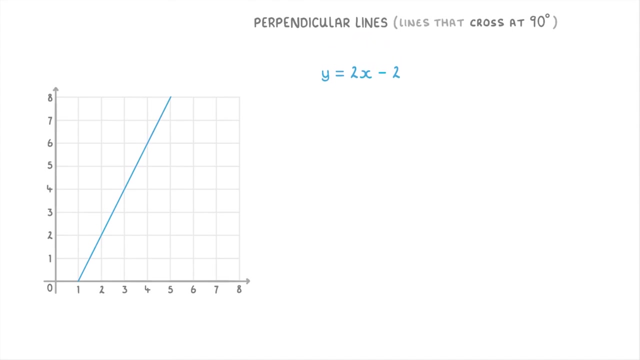 In today's video we're looking at perpendicular lines, which are just lines that cross each other at 90 degrees. For example, this line of y equals 2x minus 2, is perpendicular to. this line of y equals minus a half x plus 8, because they cross each other at exactly. 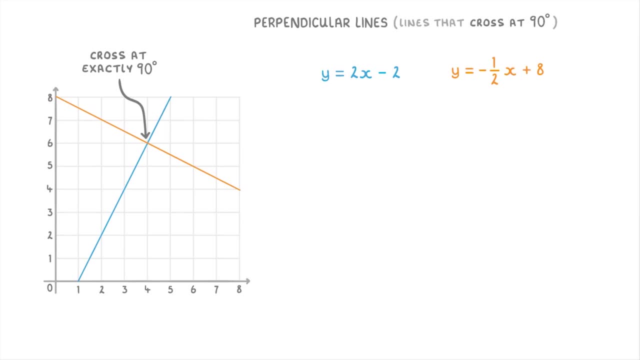 90 degrees. Perpendicular lines will always cross each other like this, and sometimes the only way that you can be sure they're perpendicular is that they will have this little square thing that indicates that they meet at a right angle. Another way you can: 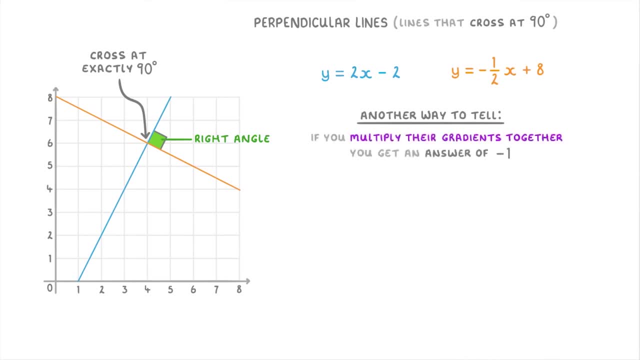 tell that two lines are perpendicular, though, is that if you multiply their gradients together, you'll get an answer of minus one, which we can show using the equation: m1 times m2 equals minus one, where m1 is the gradient of the first line and m2 is the gradient. 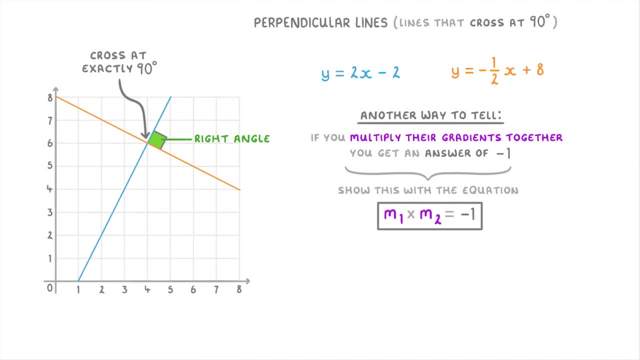 of the second line. For example, on our graph, the first line has a gradient of 2, so m1 equals 2, whereas the second line has a gradient of minus a half, so m2 is minus one half. So if we wanted to double check that these two lines were perpendicular, we'd have 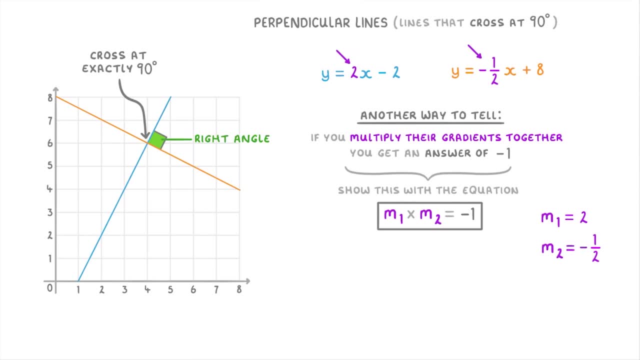 to multiply together their gradients and see if it gives us minus one. So if we give it a go, we're to just do 2 times minus a half, which indeed does give us minus one. so these lines are definitely perpendicular. Let's try and use this same idea to try these. 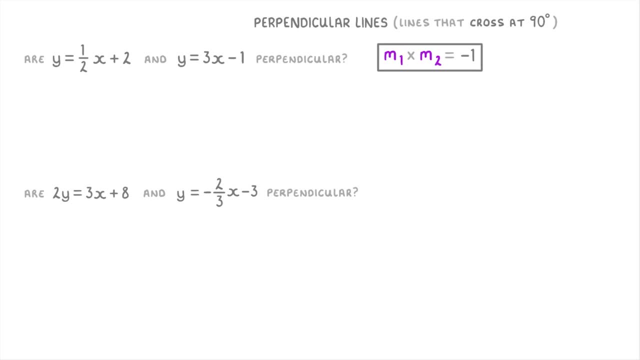 two questions where, in both cases, we're given two equations and we need to find out whether the lines they represent are perpendicular or not. So for this first question, we can see that the gradients of our lines are one, half and three, so we know that m1 is a half and m2 is 3. So to check if they're perpendicular, 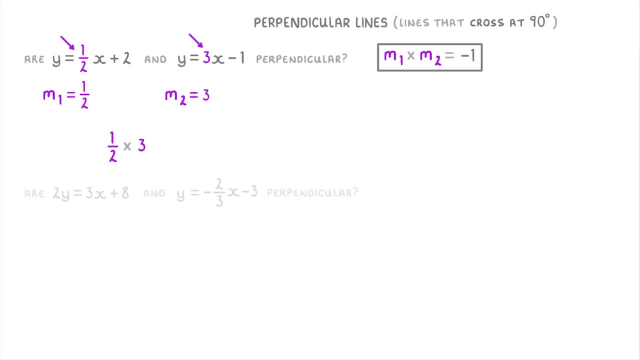 we need to do 1 half times 3, which gives us 3 over 2, not minus one. so we know these two lines aren't perpendicular perpendicular. For this next one, we first of all need to change the 2y equals 3x plus. 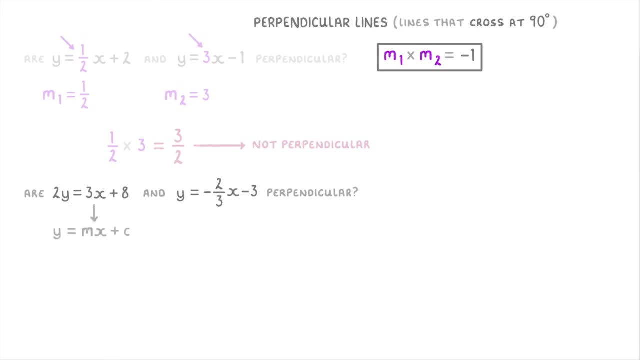 8 equation into the form of y equals mx plus c, because that will allow us to easily find its gradient. So to do that, we just divide the whole thing by 2, to get y equals 3 over 2x plus 4.. And now that we've done that, we can tell that the gradients of our lines. 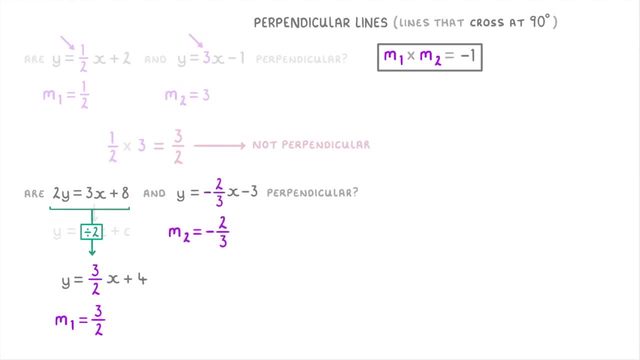 are 3 over 2 and minus 2 thirds. So to check if they're perpendicular, we just multiply these together by doing 3 over 2 times minus 2 thirds, and that gives us minus 6 over 6, which actually simplifies down to minus 1.. So these two lines are perpendicular. 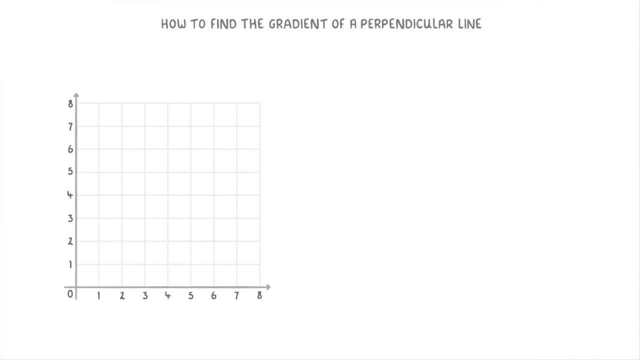 The next thing we need to look at is how to find the gradient of a perpendicular line. For example, if you were given this line of y equals 1 third x plus 3, and then told that this other line was perpendicular to it, you'd need to be able to figure out. 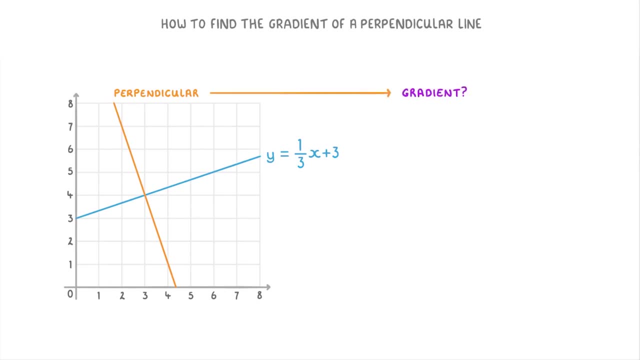 this other line's gradient. For questions like this, we can use the same formula as we were using before, but this time we're effectively looking for the m2 value because we want the gradient of the second line. So we can find the gradient of the first line by dividing both sides by m1, so that we 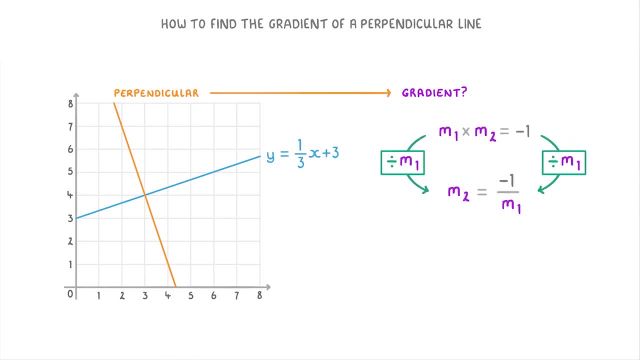 get m2 equals minus 1 over m1. Then in this case, because the gradient of our first line is 1 third, we know that m1 is 1 third, and so to find m2, we just do minus 1 over a third. 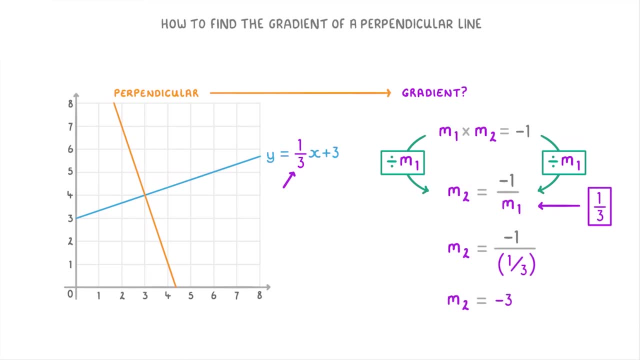 which is minus 3.. So the gradient of our perpendicular line is minus 3.. You could also be asked to find the equation of that perpendicular line, And for those questions they'll normally give you one of the sets of coordinates that the line passes.